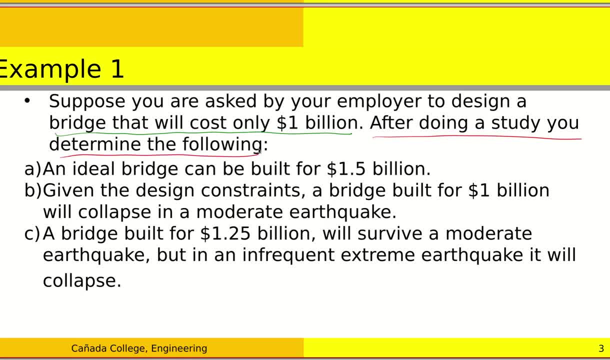 And you, along with your team, conduct a study to determine you know what you can achieve with this cost budget and you find that the ideal bridge that you would want to build, this bridge could actually cost half a billion more, So it could be 1.5 billion dollars. 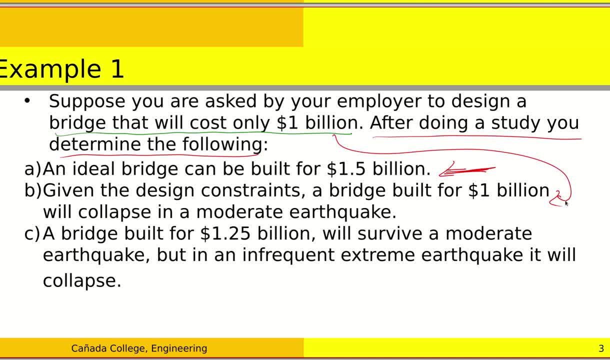 And in the constraints you're given- that is, cost of 1 billion- you find that this bridge that you build because of the constraints and cost, will actually not be able to survive a moderate earthquake. On the other hand, you see that you know, if you increase the cost to 1.25 billion, rather, 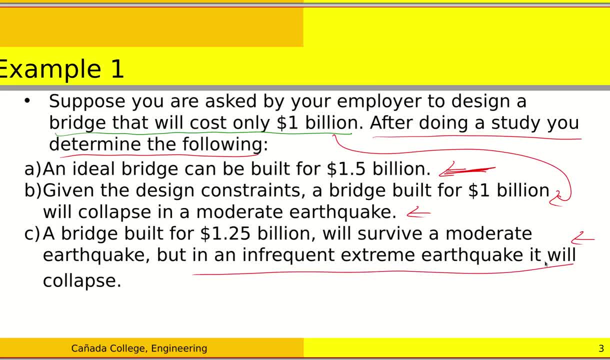 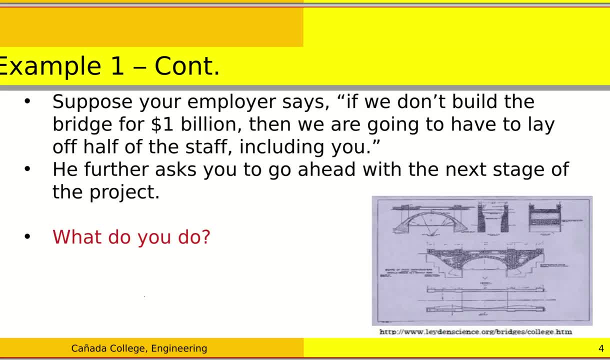 than 1 billion. This bridge can survive a moderate earthquake. If you build a bridge, moderate earthquake, but an extreme earthquake will cause it to collapse, okay, so you're, you and your team- are in this situation now, where you have these different options, so then you go back to 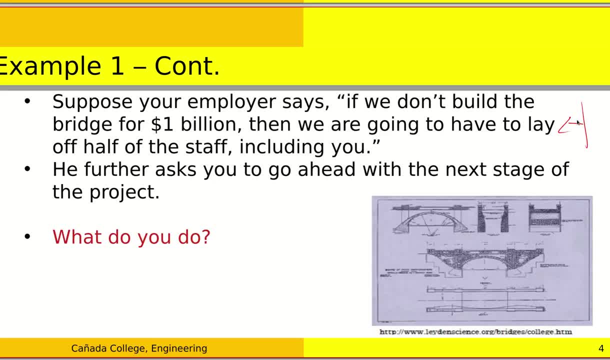 your employer and give him or her the various options. and the employer says: you know, um, we have to build this bridge for a billion dollars, because if we don't then you know we're going to lay off a lot of people in the company, including you. and he says: go ahead and get started with the. 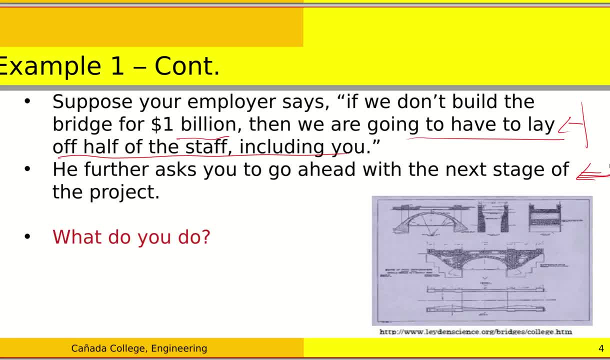 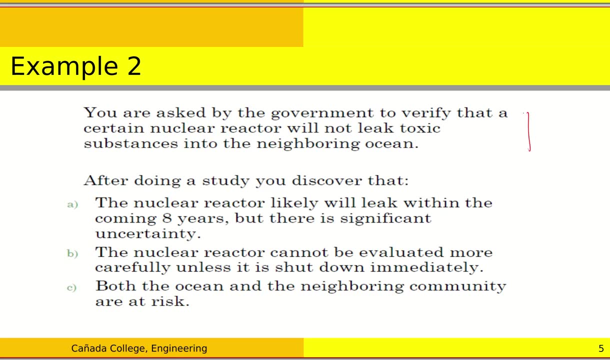 next stage of the process, of the project. right, so the question is for you, as an engineer, what do you do? so here's one example of what can happen. as an example to let's look at this scenario here. okay, you are, you know, in a government organization and they have asked you to. 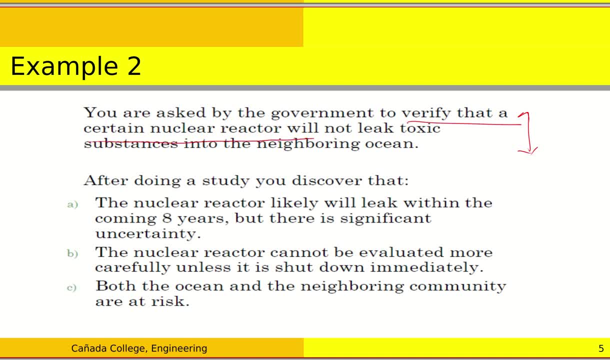 you know in a government organization and they have asked you to. you know in a government organization and they have asked you to verify that there is a nuclear reactor and you want to make sure that it does not leak any toxic material into the neighboring surrounding environment. maybe there's an ocean nearby. 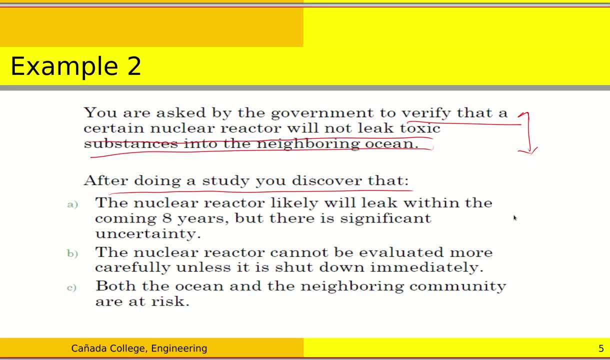 and you do a study of this nuclear reactor and you find that, you know, in the next eight years there is a good chance of there being a leak, right, but of course there there is uncertainty: it may not leak, but it might leak. and then you also find that unless the reactor is actually- uh, our reactor operation has stopped. for 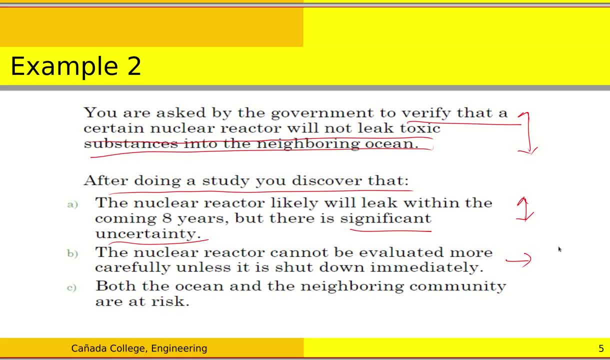 some time. you can't actually calculate with greater probability or likelihood what the consequences are, right, so you just need more information. and then you find that if the leak does occur, it's both the ocean and the neighboring community that will be attracted to by the reactor. teammate who 물 bathtub water will be glueing in to the reactor. 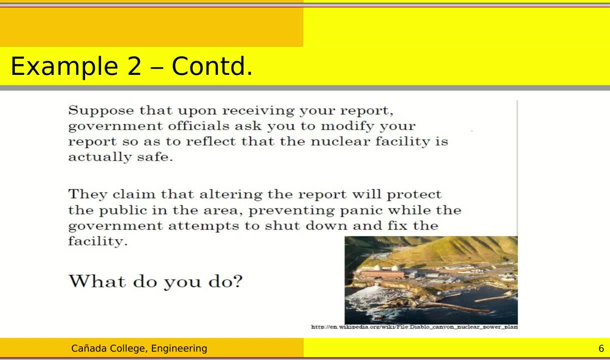 risk. and then you know, you send your report back up to the government agency and they cut back to you and say: you know what you need to modify your report so that you say that the nuclear facility is actually safe. and and they say that basically the reason that you want to alter your report is that it. 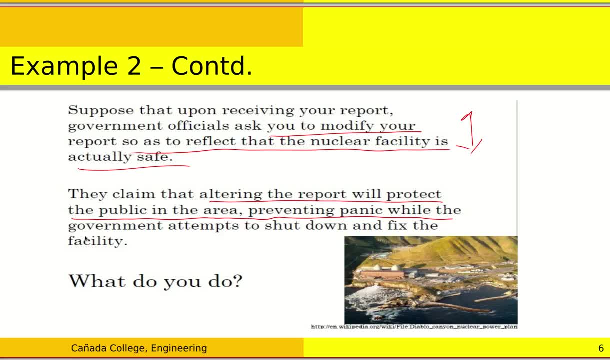 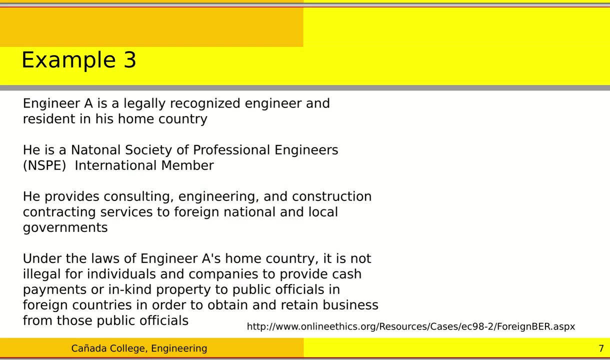 will protect the public, prevent panic and in that time frame that they have, the government will try and fix the issues. so again, the question is: what should you do? here's a third example. so let's say, engineer a is is a recognized engineer in the home country he is in. 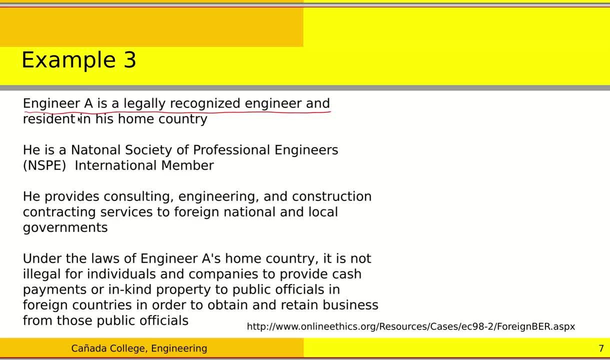 whether he's from? okay. he's also a member of the National Society of professional engineers, NSP, and he's an international member, so he is in his home country. he's able to provide consulting, engineering and construction contracting services to foreign national and foreign national and local governments. okay, under the law of the. 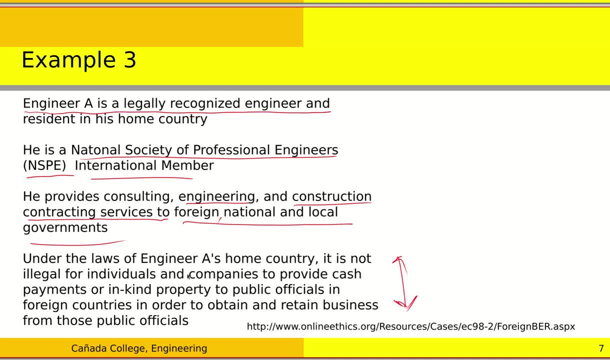 engineers, engineer at in the home country. it is not illegal for individuals and companies to provide cash payments or in-kind property to public officials in foreign countries in so that they can obtain and retain the business from these, from these public officials, right, so so we come to. 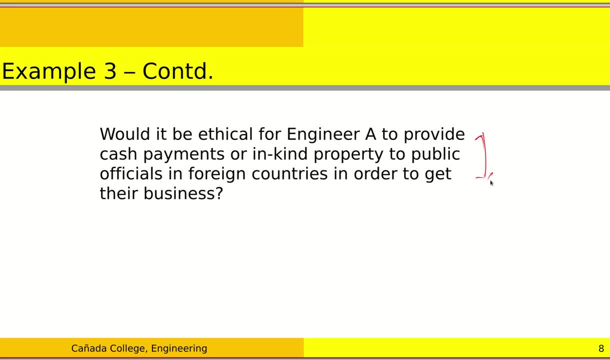 this question here, and that is: would it be ethical for engineer a to provide cash payments or in-kind property to public officials in foreign countries in order to get their business? it looks a sufficiently like a, like a bribe, right. well, so think about this. so you see that these are three examples. you've gone through three different. 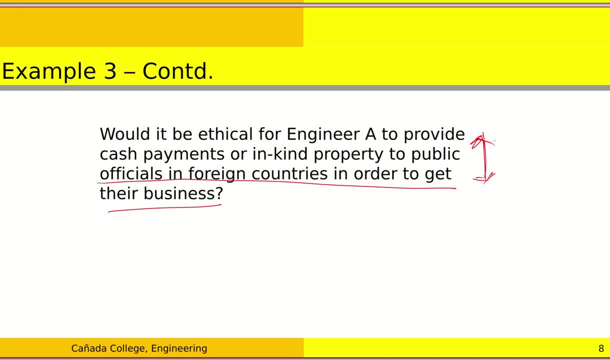 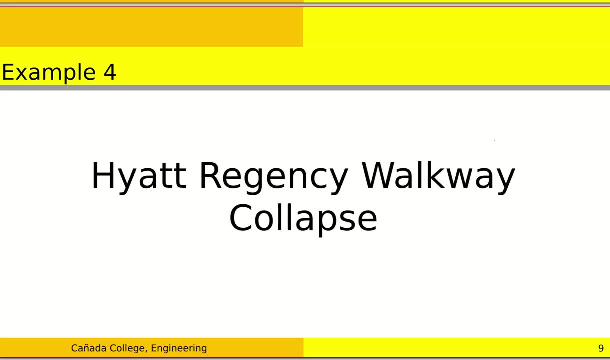 scenarios, each one, you know, leading to an important question as to whether what is asked of you is right or wrong, whether you should be doing it or not. now I'll give you an example of something that happened that has direct bearing to our understanding of various aspects of 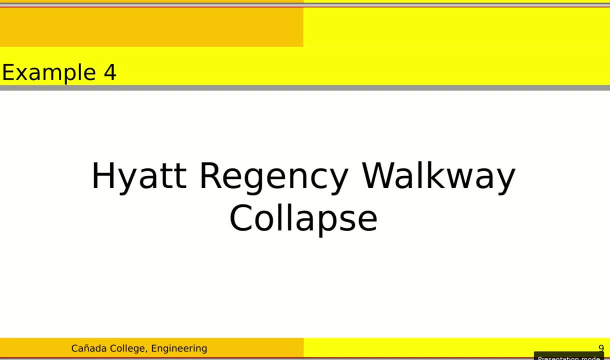 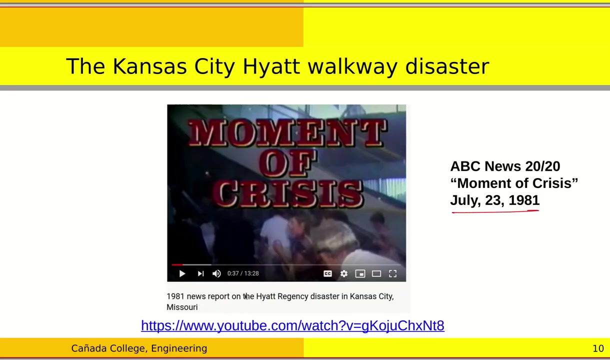 mechanical engineering or construction engineering, and it goes back to some Underlying foundations of of engineering. So this is Something that happened at a Hyatt Regency Hotel in 1981,. okay, so I'm not going to play the video here, but I would like you to go and check out this video. 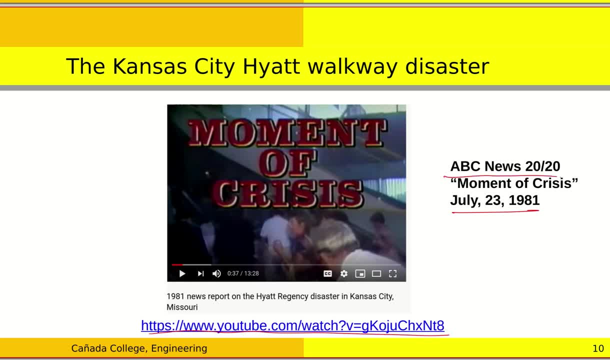 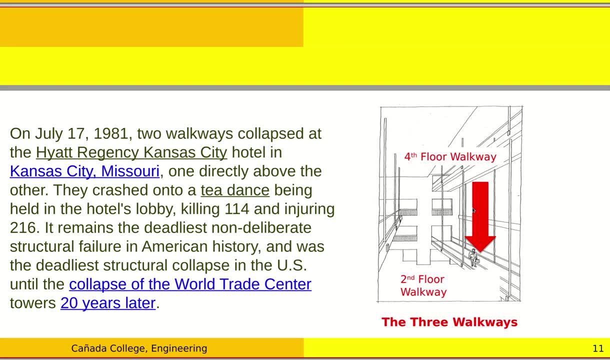 The YouTube link is provided here. It's called ABC news 2020: moment of crisis. So what happened here? Hopefully you've seen the video and then we can continue on here. What happened, as you know from the video, is that in July of 1981, 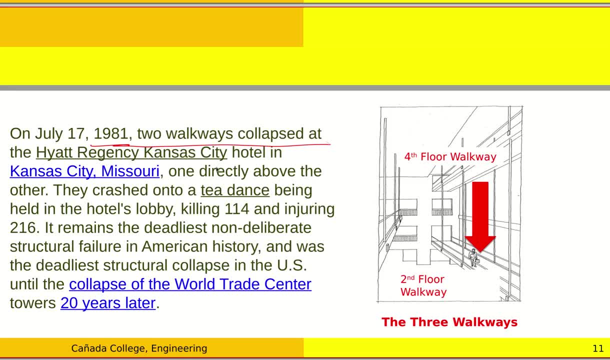 The new hotel, the Hyatt Regency, in Kansas City, Missouri. Basically, you know there was a serious disaster there where A walkway, a hanging walkway, so you can see in this image here There's one walkway here and there's a second floor walkway here and there's a fourth floor walkway here. 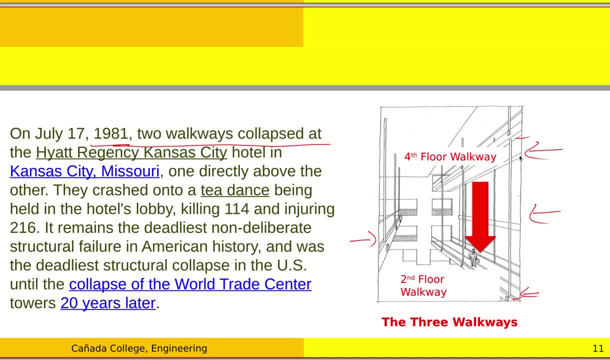 and you can see that this walkway and this walkway are connected together, but some kind of, some kind of Cable system, right? So it goes up to here. There's a gap and then it goes again. So it turns out that there was a dance going on in the hotel lobby. 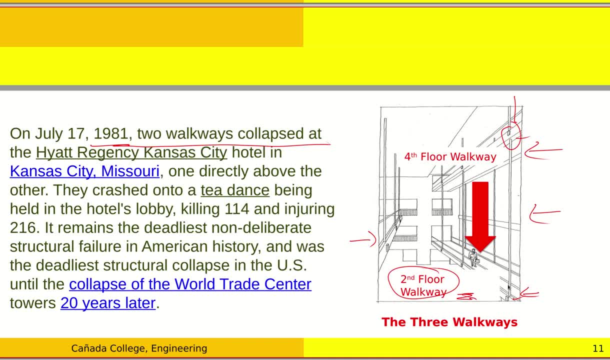 down here, and at some point during that dance- you know this- these Walkways collapsed, and it was a very deadly collapse, killed more than hundred people, and So it turns out that is still one of the deadliest non-deliberate structural failures in American history, and 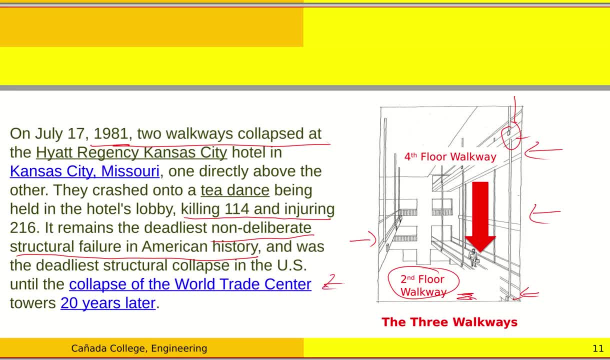 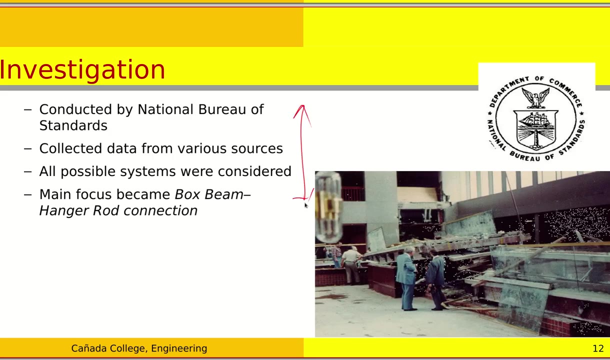 next to the World Trade Center disaster in In 1991,, I'm sorry, 2001, This was, this was. You know, this was the deadliest one. Okay, So what happened was that the National Bureau of Standards was involved in investigation of this disaster and they went about collecting data. 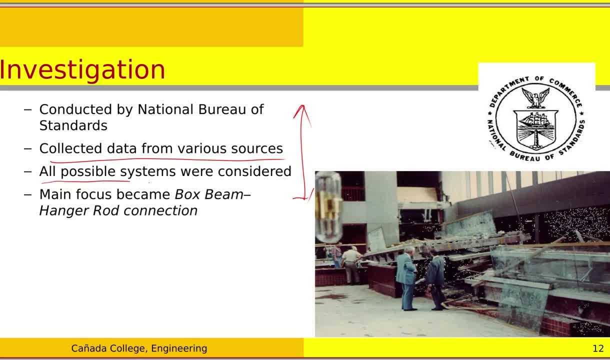 They talked to all the people who worked on constructing the building. the interviewed people who were working inside the building. they looked through all the rubble and and it turns out that this Started focusing their attention in this part of the structure here. you know this part right here. 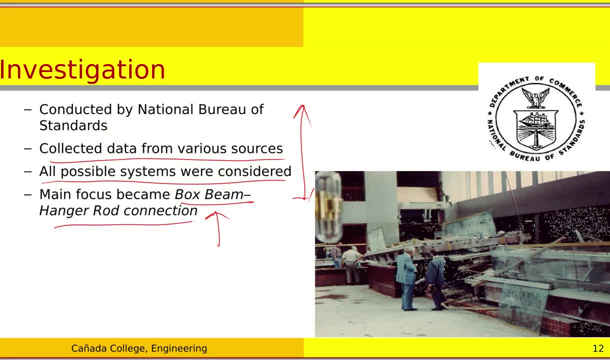 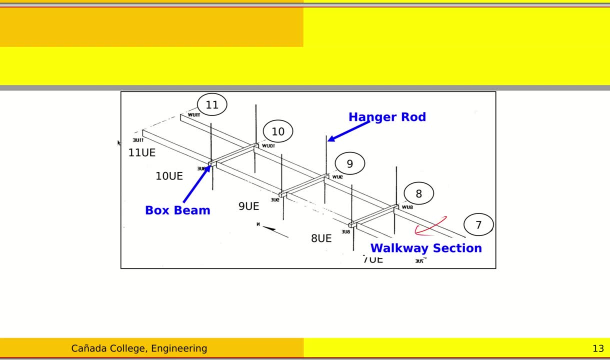 Okay, So there's a box beam hangar connection. What is that? So here is here, is your walkway section right going across here, like this: this, this part here. So that's your walkway section and that is being supported By this cable system. So what I highlighted earlier, so you have cable go up here and 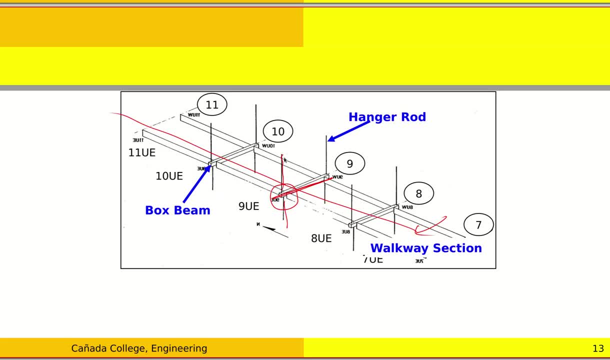 There's a box beam and then on the cable That is, you know, hanging it up or holding it up, And so you had this periodic box beams and The cables that are holding it up, as well as cables from the lower lobby that are, you know, being attached to it. 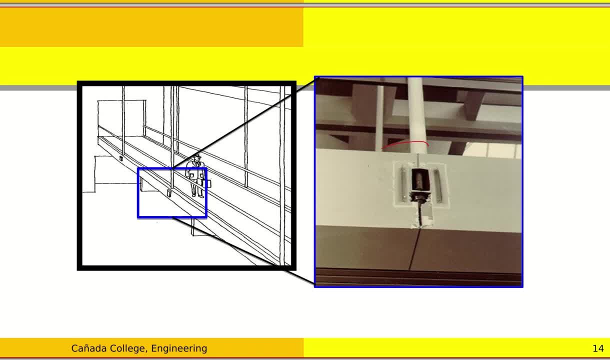 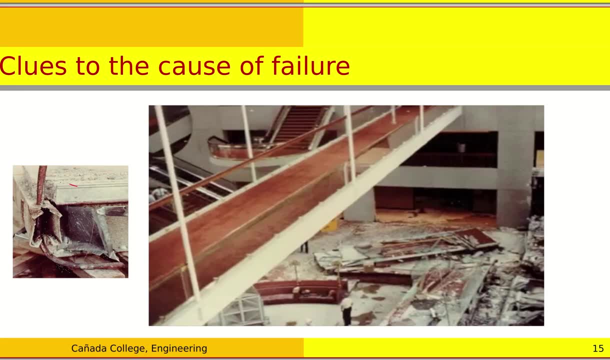 So here's what it looks like And here's the real-life image of it. Yeah, so When they looked into the accident, they found that, you know, they had striking evidence that whatever happened originated from this area where the cable was attached to the box beam and. 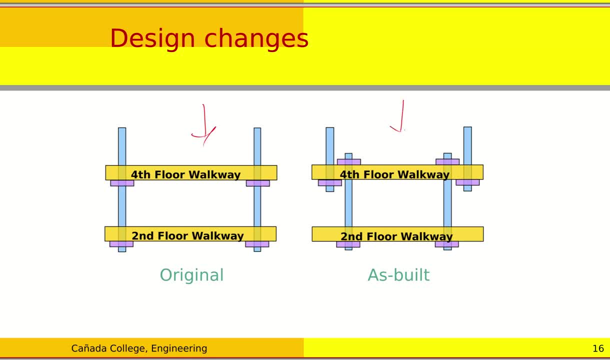 Then they went and looked at the design that was originally approved and the design that was actually implemented. so this is what the original structural engineers had designed for the building and This is what was actually ultimately used to construct the, the walkway. now, without going into details, it turned out that 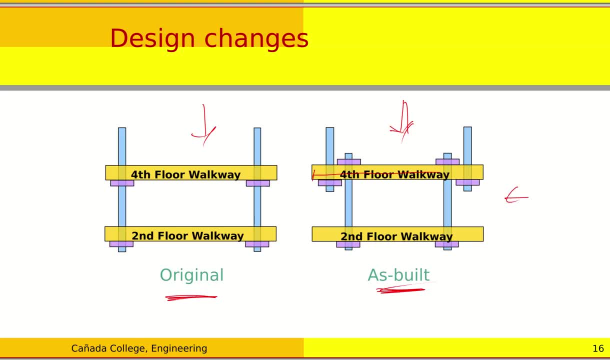 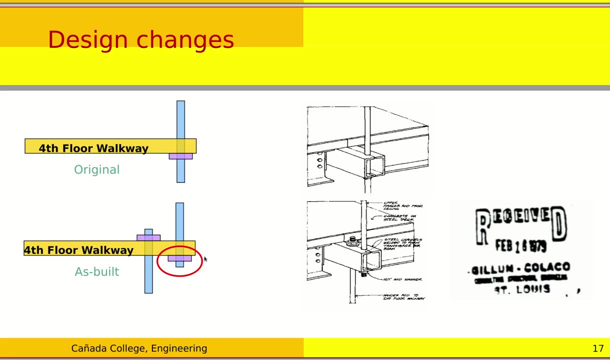 this design here actually substantially increases the load on the fourth floor walkway because now it has these two joints here at each end, as compared to this case here, and this turned out to be a fatal design flaw, right and, and so here is this. you know the, the engineering company. they basically 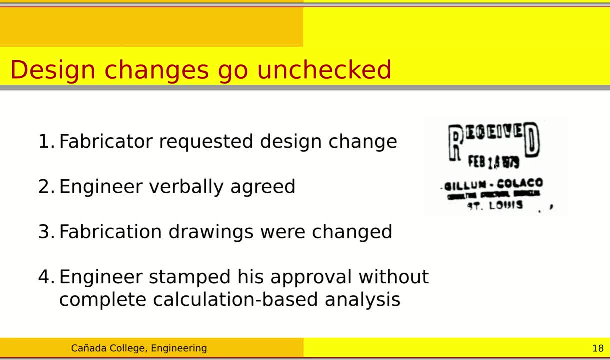 approved this design without doing a thorough calculation. so here's what happened. the installer, the fabricator, requested this design change. the engineer verbally agreed to it. they changed their drawings and the stamp their approval. but this approval is without a complete calculation of what is going to happen to the load and 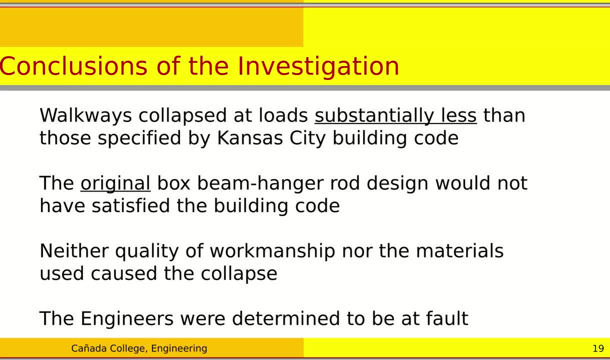 whether it was going to be able to take that load or not. so it turned out that, from the investigation, this walkway collapsed at loads significantly lesser than what was specified by the building code for Kansas City, and and so this, this, this design did not satisfy the building code. okay, the one that was used. 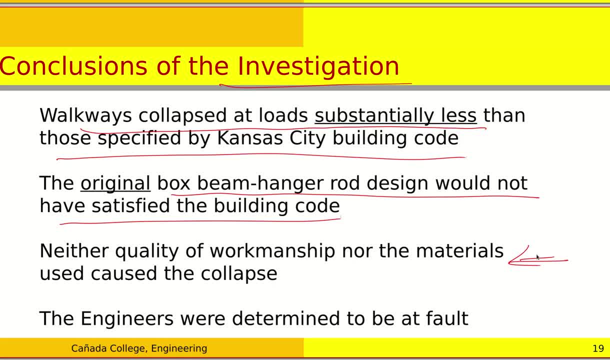 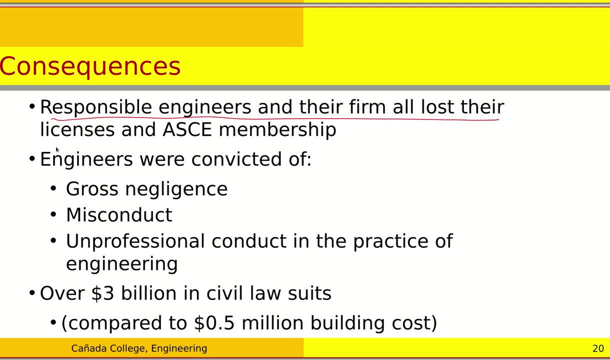 and so, and it was nothing to do with the materials used or the quality of the work done, and basically the blame was that the engineers did not do the job properly. it's a consequence of this was that all the responsible engineers and the firm that was involved- they lost their 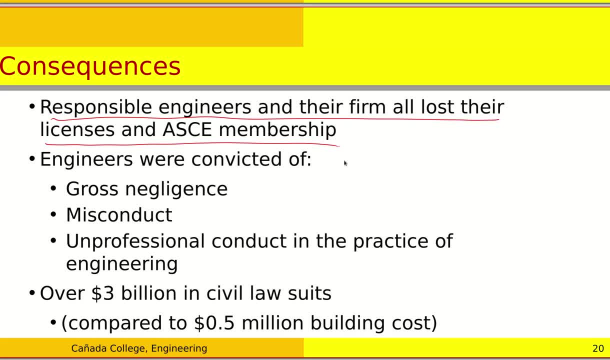 licenses. and and of course, there was the lawsuits filed- over three billion dollars in civil lawsuits compared to the cost of the building, which is half a million dollars. and so the engineers were convicted of gross negligence and misconduct and unprofessional conduct in the practice of engineering, and so 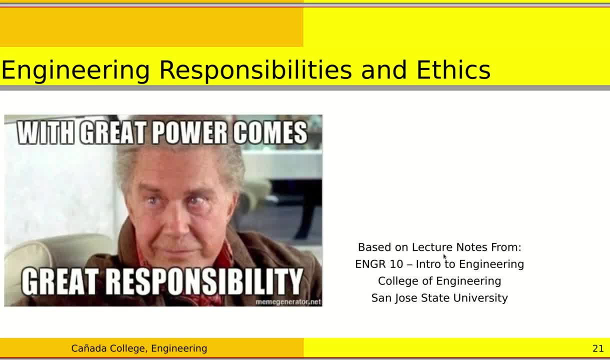 they never again were allowed to practice engineering. so so the point is that as an engineer you have great power, and so with that comes great responsibility by way. so this is famous line from the spider-man movie, which, as you know, has some very interesting engineering technologies built into it, such as the spiderweb, which has a lot of strength and she loves to. have alongside all the different structures in it, and we can find so. so in the infinite filtral and everything, basic things. it's pretty simple and we call this: does anything you have to set aside any of jobs to find, in case oflocks, in the best industry, a juror? see the absorbs соб ie, you must call because you know the Hello, I know that this word when it is important. 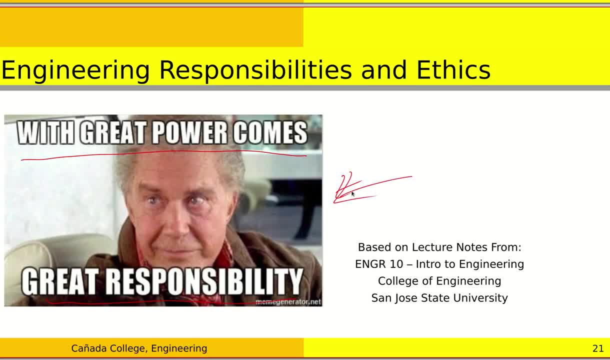 and so you know it's a, it's an interesting material to to look at from from the viewpoint of strength to weight ratio. so anyway, so point here is that the reason we want to understand, you know, you know our responsibilities is because ethics is fundamentally important to the practice. 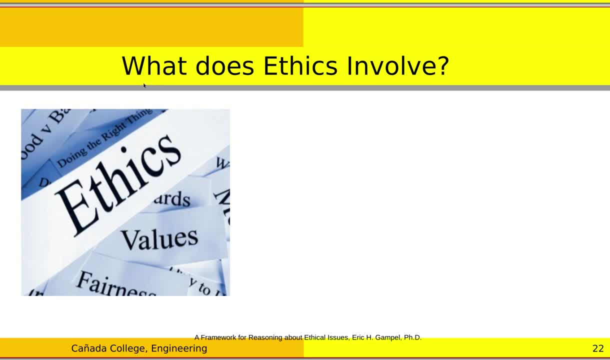 of engineering. okay, so let's begin with this question. you know what is ethics. what does ethics involve? right? well, ethics basically means, or involves, investigation of you know what is right versus wrong, what is just versus unjust, it's good versus bad, virtuous is wise. so these are the things that you know as an engineer. you're constantly balancing out in the context of 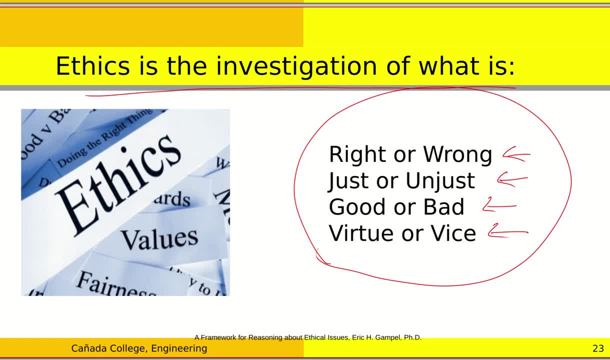 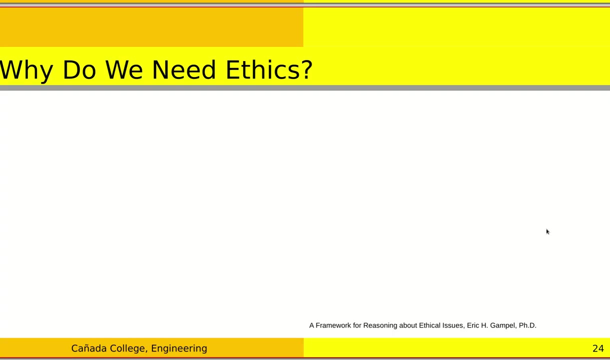 you know solutions you might be implementing to solve a pollution crisis, a traffic you know, a highway crisis or any other activity that you're involved. these are going to be part of your design process, part of your implementation process. so the reason we want ethics to be guiding our decision making is that, on one level, it 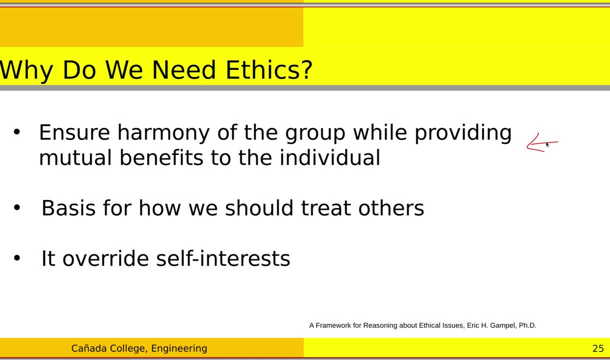 um ensures that whatever we do, we're not going to be doing anything wrong. so we're not going to just do anything, but do something to be done with it. it doesn't have to be successful right. regardless of the own, my own belief, which is just human, life science has a clear purpose. 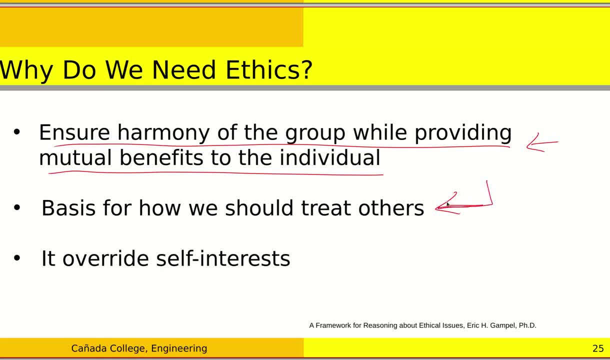 so it's just mind for the sake of focus and it's Dang. they don't have your deepness level right. and so I think, when we think about ethics in our thinking and ability to think on the right planning basis, we see the &, D & P outer cost to practise their objectives. Nacho. 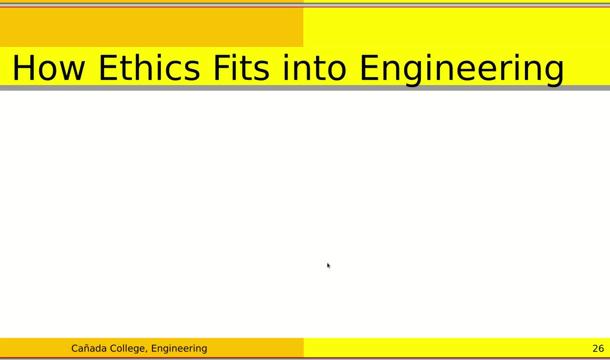 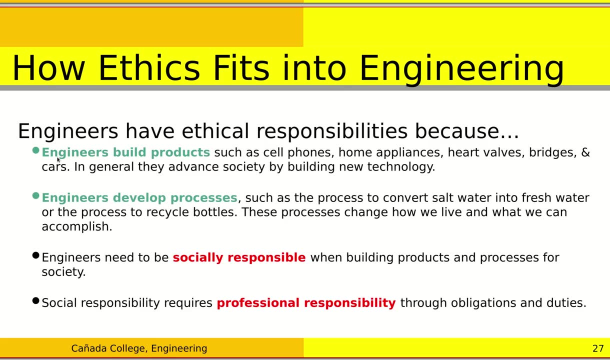 which is the right strategy. we take care of it. pulp out the core of our recommendations. as you know, an engineer basically builds products. right, they develop processes and so, in the context of this, we just take the example of building products- think about cell phones, home appliances, bridges, cars, you know, biomedical devices. they're basically advancing society by by these new 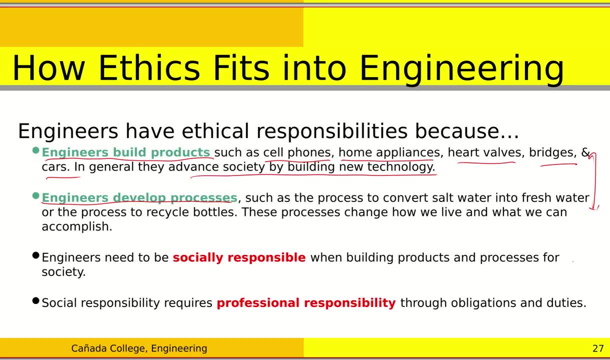 technologies and all of these new technologies, you know, when you start thinking about making them, you want to start thinking about being. you know, how does my manufacturing of this particular product affect society? well, on one hand, society probably gets direct benefit of, you know, having a heart valve or building a bridge. but what does it take to build that? you know, am i consuming? 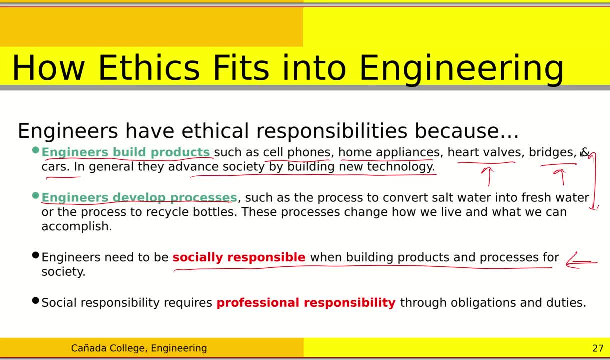 resources that are basically very scarce. am i polluting the water in my house or in my house around my factory? am i spilling a lot of greenhouse gases when i'm in from my from my factory? so these are the things that we have to take into account as an engineer right, and similarly when you develop. 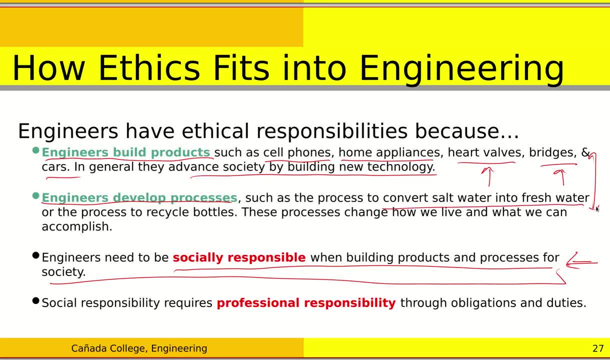 processes, for example, when we are creating drinking water from salt water or recycling bottles. again, these are things that have impact on the society in terms of human impact as well as environmental impact, right? so ethics is uh is integral to the operation of an engineer, right? and not only are engineers required to be socially responsible, they're also required by 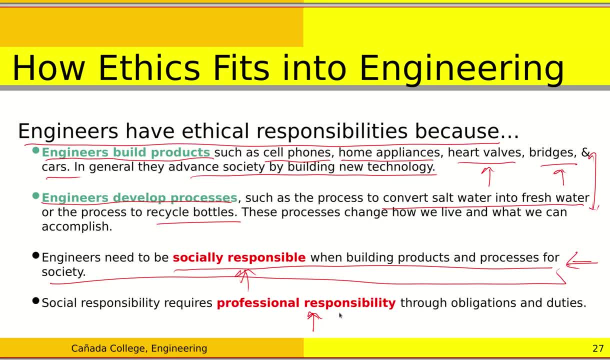 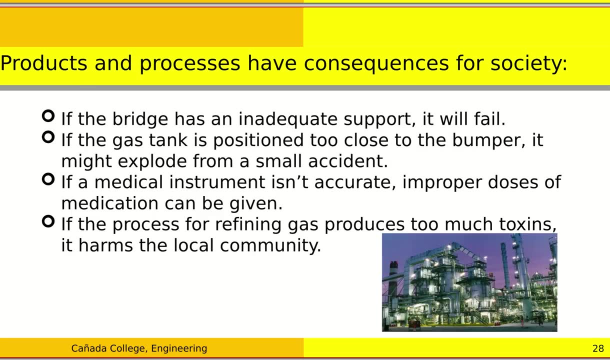 their own profession. depending on whether you're a mechanical engineer or civil engineer, you are required to be professionally responsible to your, to your engineering field as well, and this comes through through various obligations and duties that that you have to take into account when you that you are tasked to do so. just thinking about, you know, reiterating the idea that any product that 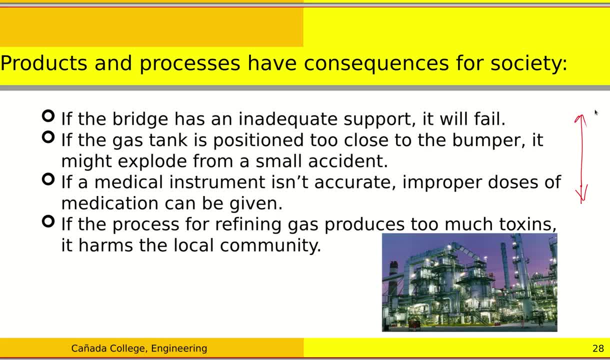 we make has a consequence and society. many times it's designed to have an intended consequence of benefiting society, but sometimes it has the unintended consequence that it might actually produce harm to the society. who knew that when plastics were invented that there would be such a major cause of harm to the society? and so i think it's important to think about that, and i 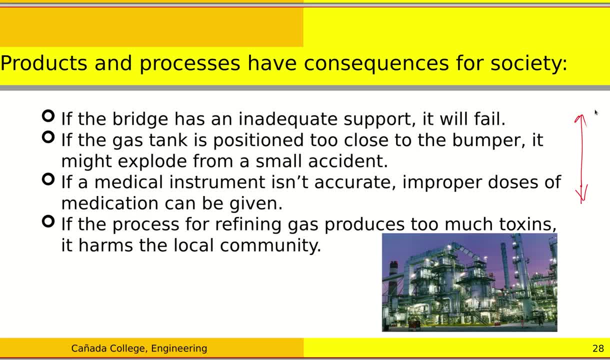 would like to thank you for your time today and i hope to see you soon and i wish you all a great weekend and i wish you all a very happy work day. thank you, um, uh, understanding of okay, is this really good? are the benefits going to significantly outplay? 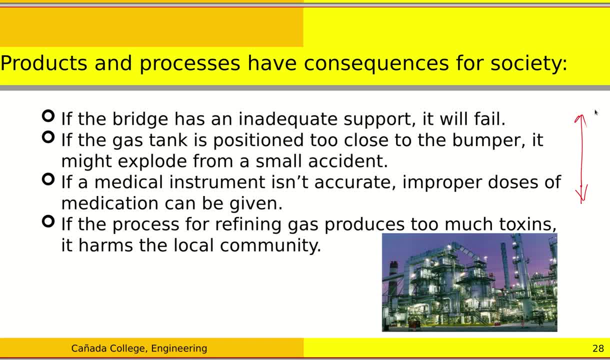 um, the the negative impacts, and what are these negative impacts and how do i mitigate them? right, so, those are things that we have to constantly think about. you know, here are things that have direct consequences, right? so, if you build a bridge and it's not designed properly, 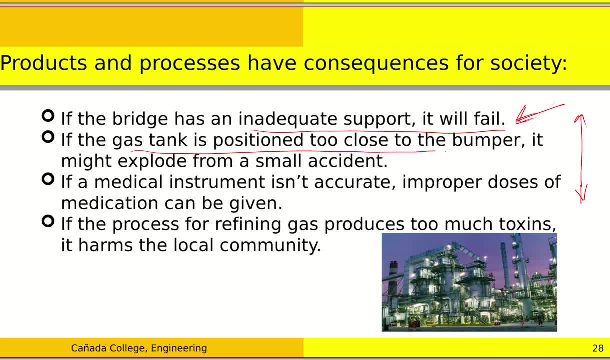 it's likely to fail. if a gas tank is positioned too close to the bumper, it might explode from a small accident. uh, medical instrument isn't accurate, you know. it's not giving the right dose. it might actually cause harm. refining gas produces too much toxins, and so are these toxins. 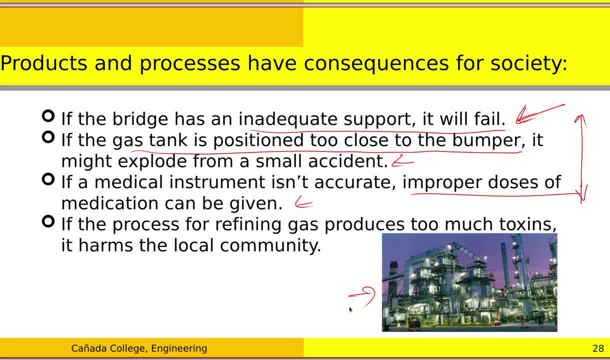 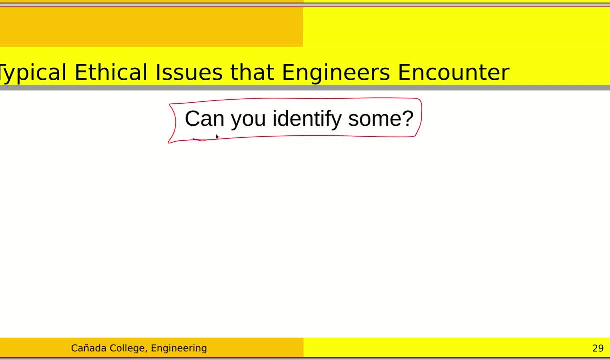 being sent out into the community or are they being captured and recycled in some way? so, uh, so you know you should take a moment here, you know, spend you know five or ten minutes and just kind of think about your role as an engineer, you know, think about you being in an engineering organization. 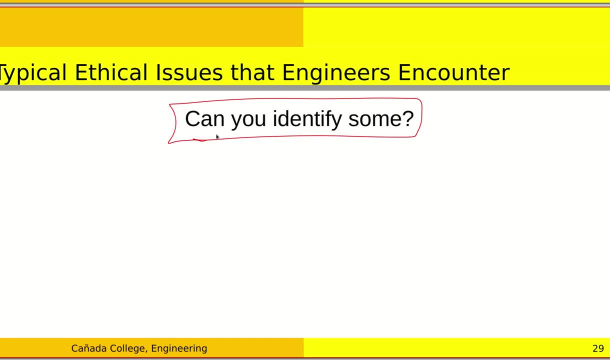 and just start. you know from day one that you enter the company. uh, what is it that you think you're going to be doing besides? just what you think is engineering, which is, you know, creating new products, solving problems, things that, as you will see very quickly, every discussion, every. 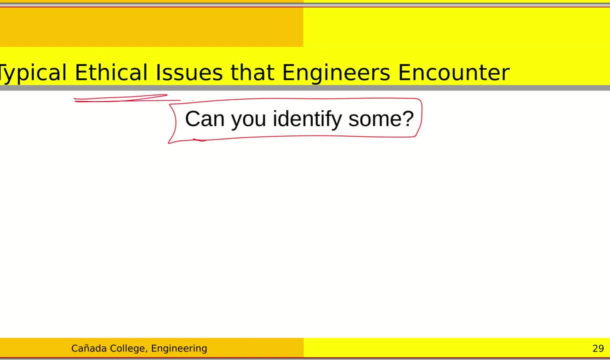 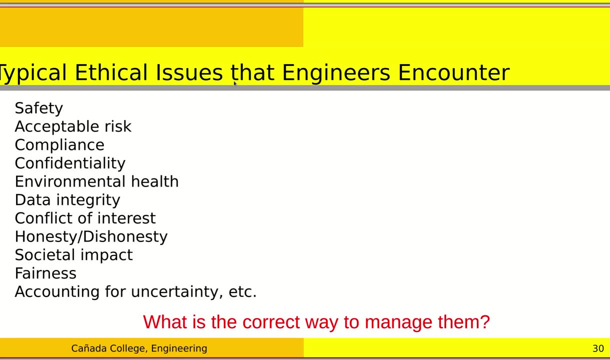 you have will be, uh, in the framework of trying to make sure that whatever you do is ethical. okay, so here are some, a list of some things that you know you would be thinking about: safety. what is acceptable risk? is it compliant with the, the rules of, of the, of the um, of the? 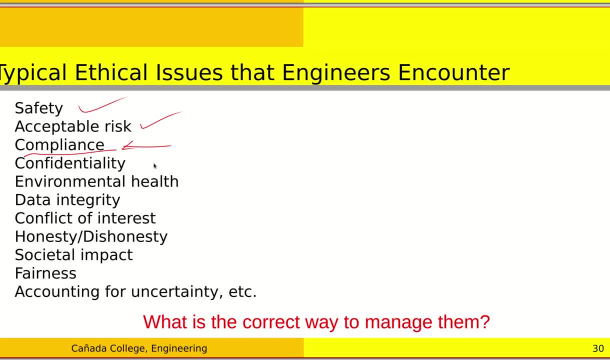 local society that you are going to be implementing this uh solution in. uh, you know, confidentiality, environmental health, uh data integrity. so these are all aspects of ethics that are going to be involved in your activities as an engineer, right? and so what this topic is about is: how does one go about um managing these issues, these ethical 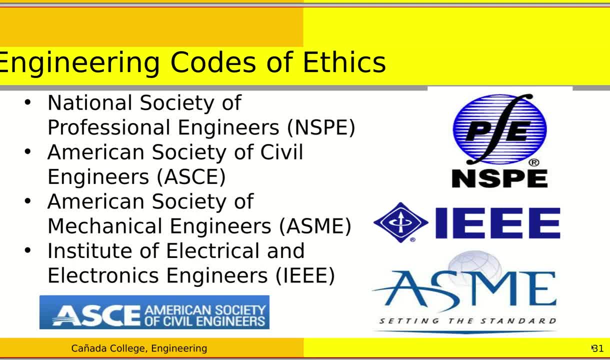 issues. okay. so the good news is that at the outset, as we start getting trained as an engineer, we are going to, of course, look at ethics in engineering classes, but also as you become a professional engineer, you will see that the various societies that you are part of you know, for example, the american society of 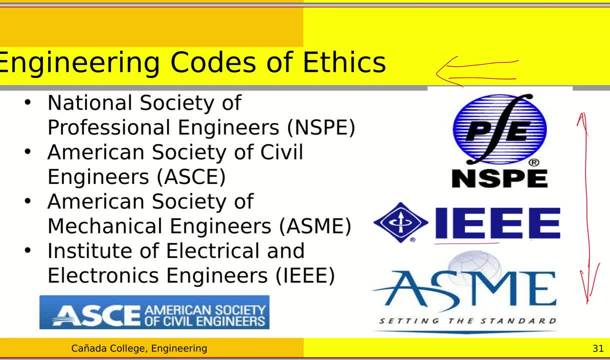 mechanical engineers, or the institute for electrical and electronics engines, ieee, or the society for civil engineers, asce national society of professional engineers. so all of these have clear engineering codes of ethics. okay, so that means that there is a, there is a document, there is a, there is a book that tells you what are the codes under which a mechanical engineer is going to. 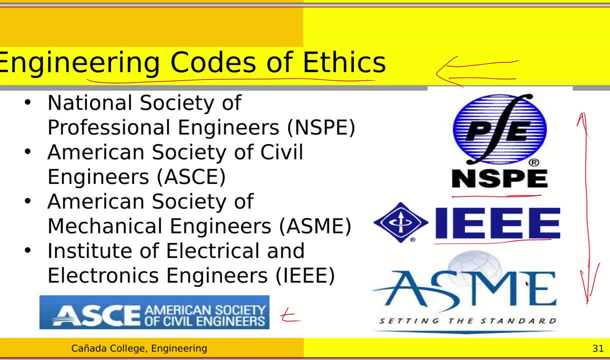 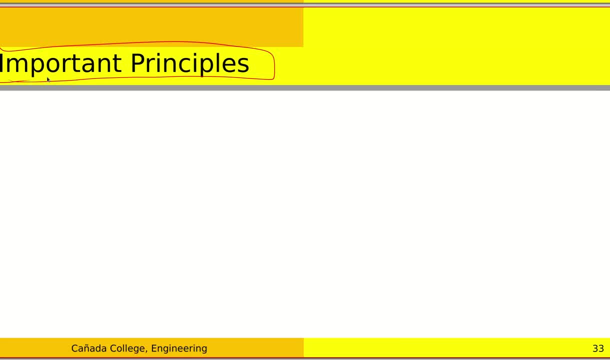 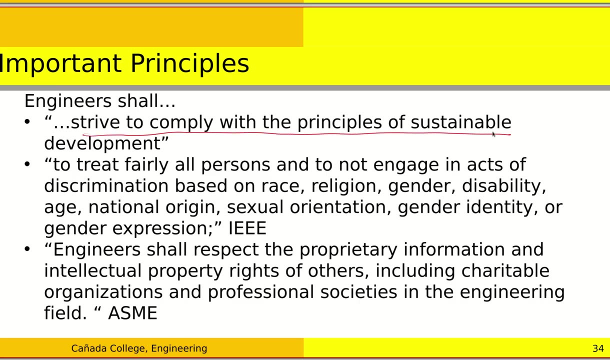 is going to carry out her activities as part of the profession, right, and? and so let me kind of give you a sense of how these codes arise. it begins, at the highest level, by some important principles. you know, these are things that many of us recognize. you know, for example, an engineer shall strive to comply with the principles of sustainable. 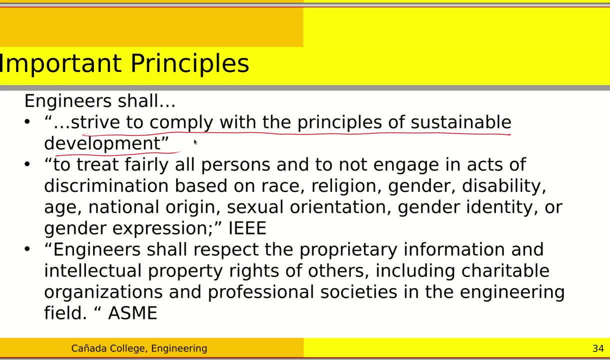 development. so in today's environment it makes a lot of sense to think about this because we want to make sure that we are. we are trying to reverse, if not improve over uh over the past generations by not making major impact environmental issues. we have a lot of principles of sustainable development. 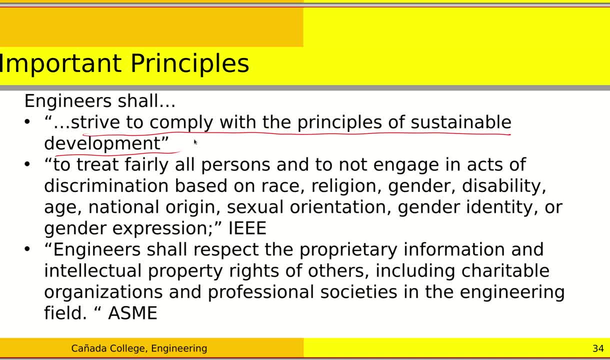 negative impact on on the environment. secondly, engineers will treat fairly all persons and will not engage in acts of discrimination based on race, religion, gender, disability, age, etc. right, and this is one of the principles in the in the IEEE ethical code. similarly, ASME says that engineers shall respect the. 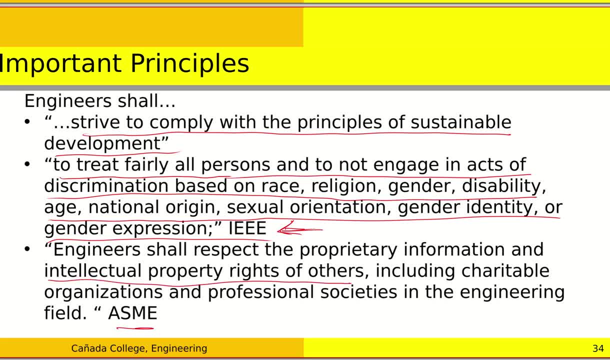 proprietary information and intellectual property rights of others. that means we are not, you know, cheating by taking ideas from others without giving due recognition. right, you are welcome to take the idea of another, but you have to compensate that organization or the person right and not not make it sound. 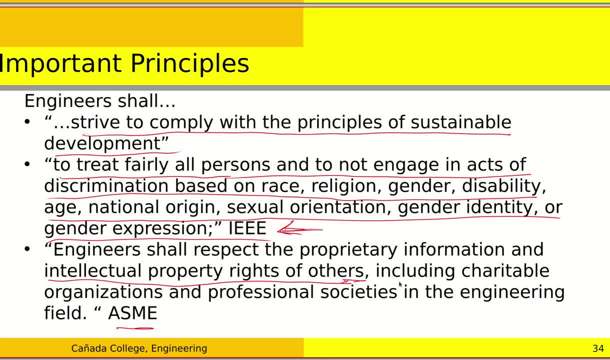 like, you created the idea and, and, and try to cheat the other person out of the fact that they were the ones who originally created you know the new idea, right? and so these are some important principles that guide all engineers, right? and so these are some important principles that guide all engineers. 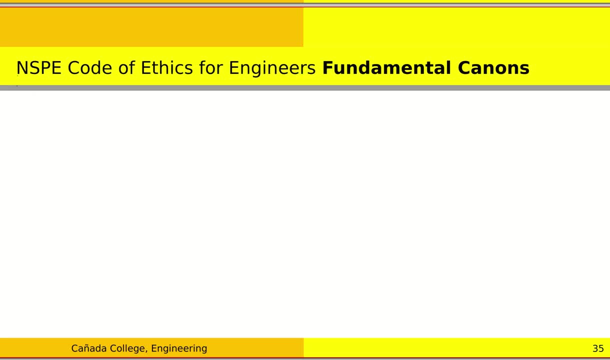 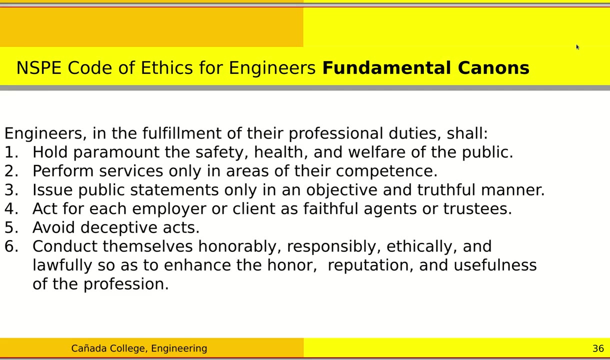 And it turns out that the National Society of Professional Engineers has put together what is called the fundamental canons for the ethical activities of engineers, and these are the following: There are six of them, And so, as an engineer, as part of your professional duty, you should hold paramount the safety, health and welfare of the public. Perform services only in areas of your competence. That means you should be trained to be able to do what you're doing, or you have experience with doing what you're doing. 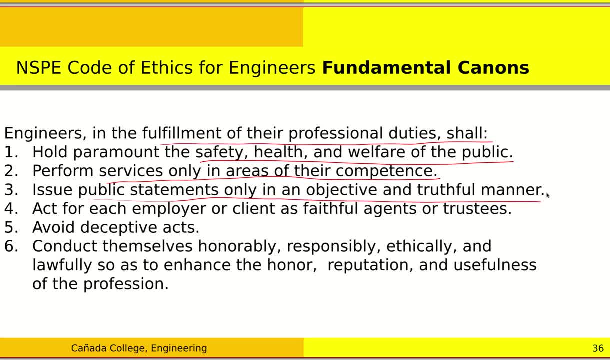 Issue public statements only in an objective and truthful manner, Act for each employer or client as a faithful agent or trustee, Avoid deceptive acts and then conduct themselves honorably, responsibly, ethically and lawfully, so as to enhance the reputation of the profession. 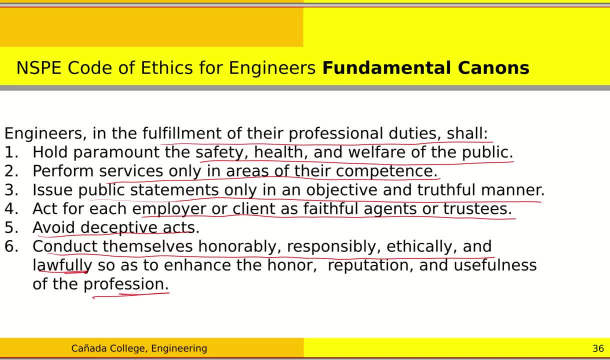 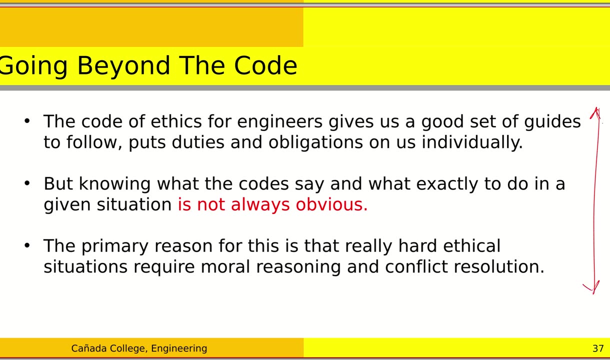 So, as you see, in these six canons, one of them is to really make sure that if you're a civil engineer or a mechanical engineer or a materials engineer, you're actually looking out for the profession by doing your best job at it, So you know. so this is a starting point. You first understand the codes and then the next step is to learn to apply them. 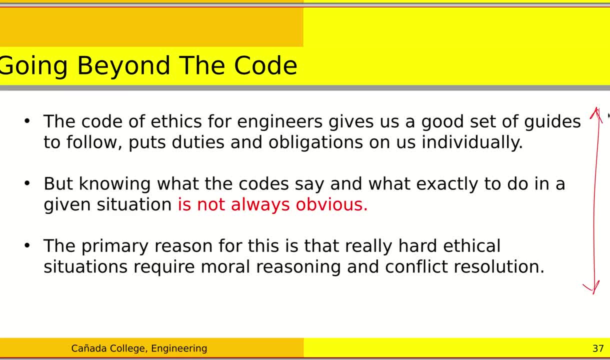 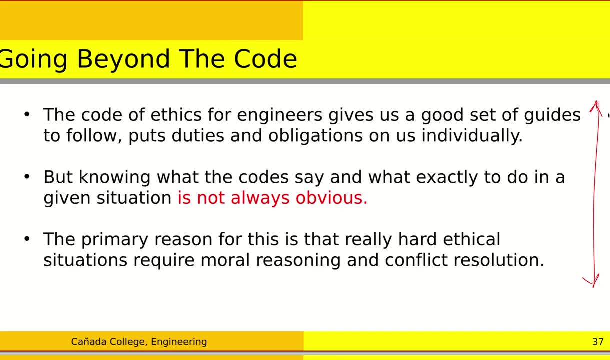 You know we started this lecture with three examples. In the next lecture we will actually go back and look at you know how- to how to actually decipher what we should do, because you know knowing the codes is one thing but it is not obvious. you know how you want to implement those various aspects for a given situation. 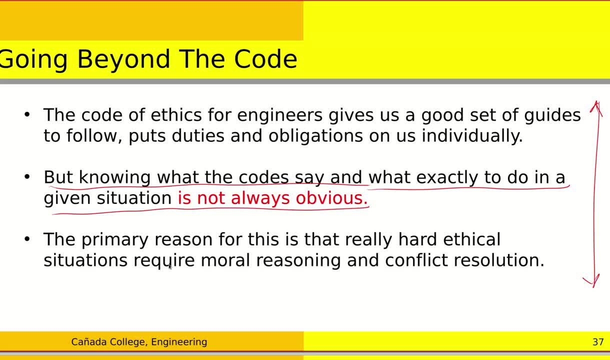 Right, And the reason for that is that, although we have these good set of guides to follow, sometimes you know the question that is posed is a really hard ethical situation and goes beyond the codes here, because it requires you to to introduce moral reasoning and a form of conflict resolution to really come up with a good, good response. 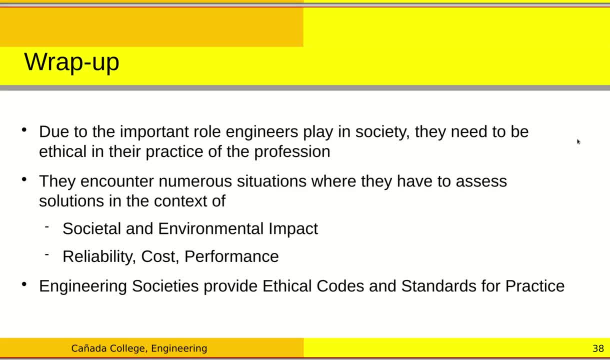 Right, And so that's what we'll do in the next class. So today, just to wrap up, I want to emphasize that, since you, as an engineer, play a very important role in society, ethics is fundamental to the practice of the profession.